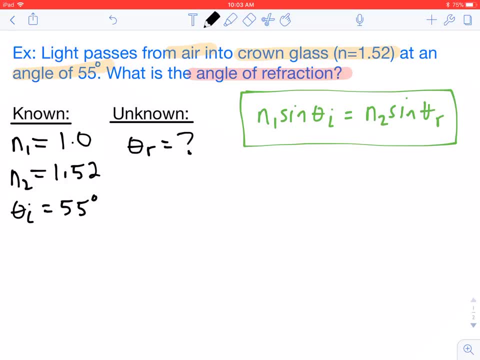 If you take a look to your right in the green, we have the Snell's Law equation. So at this point we're just going to start plugging in our values into the equation. We have to keep in mind that we don't know. theta R. 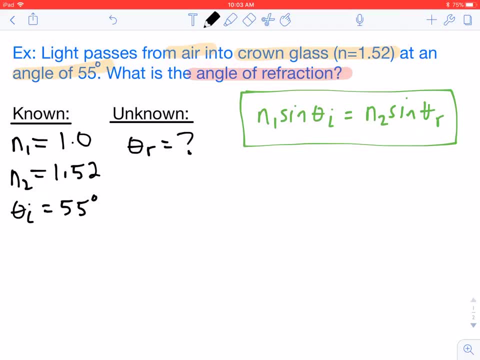 We have to keep in mind that we don't know theta R. Keep in mind, though, that when we use this equation, that your calculator is in degrees mode and not radians mode. So, first off, N1 is 1.0, sine of theta I, which is 55 degrees. 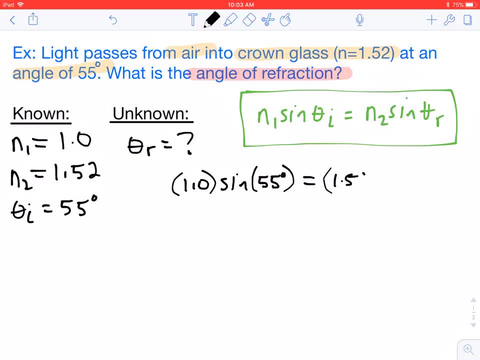 That's going to equal N2, which is 1.52 times sine of theta R. So our goal is to get theta R all by itself. So the first thing that we have to do here is divide by 1.52.. 1.52 on both sides. 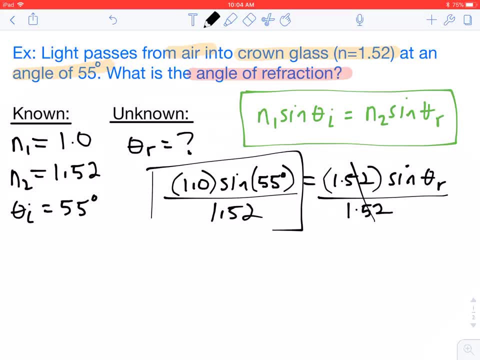 And when we do this calculation you can plug all of this into your calculator all at once. So sine of 55 degrees times 1, divided by 1.52, gives us an answer of 0.539.. Now this equals the sine of theta R. 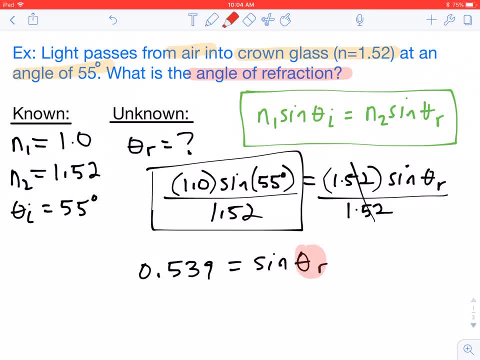 Now remember, we're going to use theta R. However, we're trying to get just theta R all by itself. So we have to figure out how to get rid of this sine function. Well, if you know your math, then you know to get rid of the sine is to take the inverse of the sine. 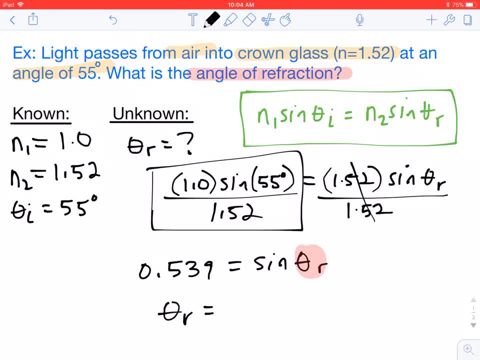 So to get theta R all by itself, what we're going to do is we're going to take the inverse sine function. So it looks like this: sine to the negative 1. There is a particular button on your calculator where you can just hit. 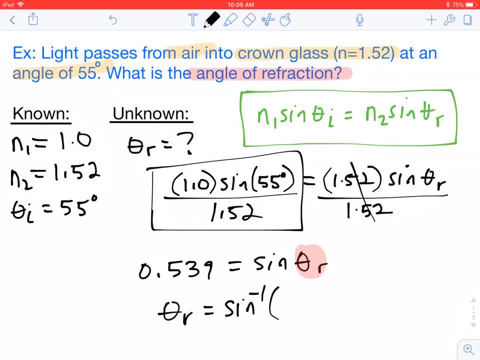 The inverse sine function And we're going to take the 0.539, take the inverse sine of that. That is what's going to give us our angle measurement. So in this case, our angle measurement comes out to be 32.6 degrees. 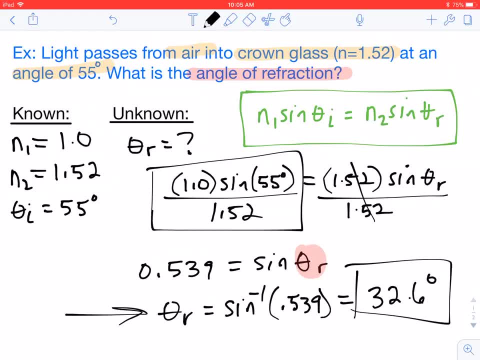 Okay, This last step, right here, of taking the inverse sine. that's usually the hardest step. It's kind of this one additional step that students Tend to forget. So make sure that you don't stop at this step. Do not stop here. 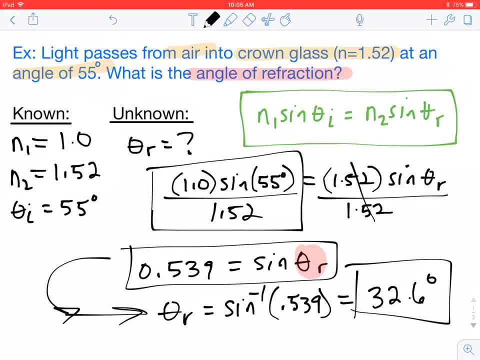 Go down and make sure that you take the inverse sine of your decimal. Hopefully this helps you solving your own Snell's Law problem. And, as always, thanks for tuning in.